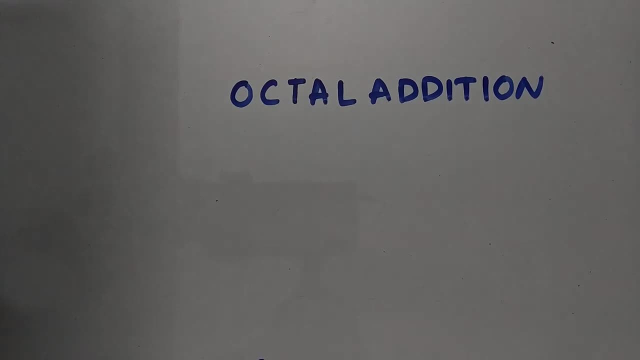 hey guys, welcome back to another interesting topic. so today's topic is about octal edition. so before going to octal edition, can you please click that subscribe button so that we can get connected and I will answer all your doubts within 24 hours if you comment down below. so without any further delay, 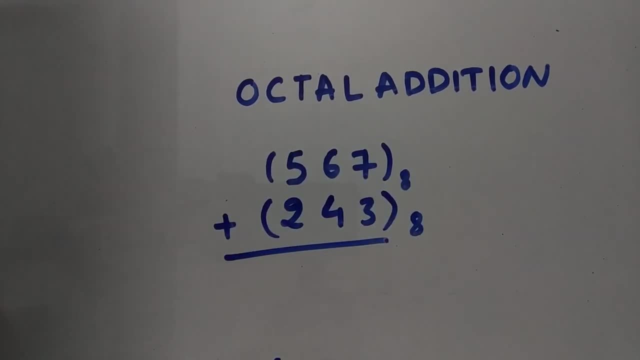 let's go into an octal edition. so I got a simple example for you here: five, six, seven, base 8, 2, 4, 3, base 8. now let's add them: 7 plus 3 is 10: 0, 1. carry over here. 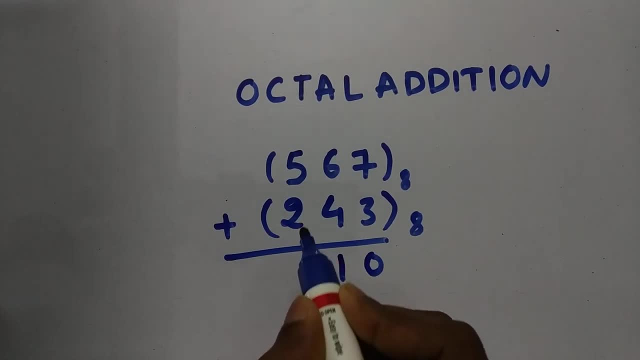 6 plus 4 plus 1 is 11. 1 carry over here: 5 plus 2 plus 1 is 8. this is not how you do. octal edition: this is decimal edition of base 10. okay, so this is of base 10 we. 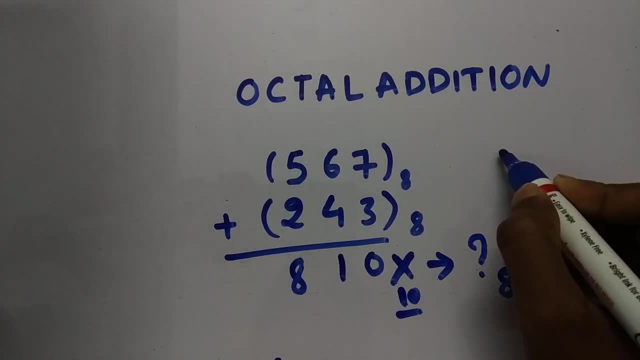 need to do in base 8. you know the base 8 has values from 0 to 10, so we need to do in base 8. we need to do in base 8. you know the base 8 has values from 0 to 7, don't forget it. base 8 has values from 0 to 7, so we need to convert whatever. 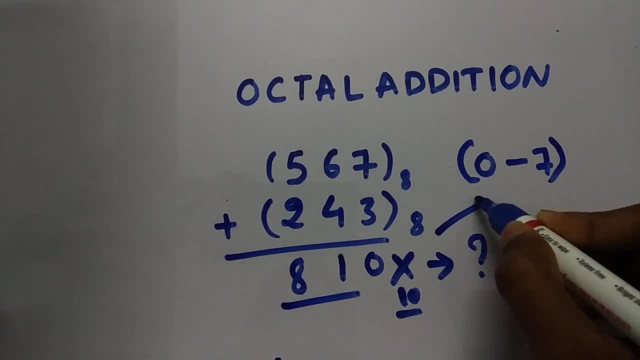 results we are getting in decimal we need to convert into octal. so whatever we are doing, addition can be in decimal but the results must be in octal. so whatever get, we get the results over here: 7 plus 3, 10. we need to convert that. 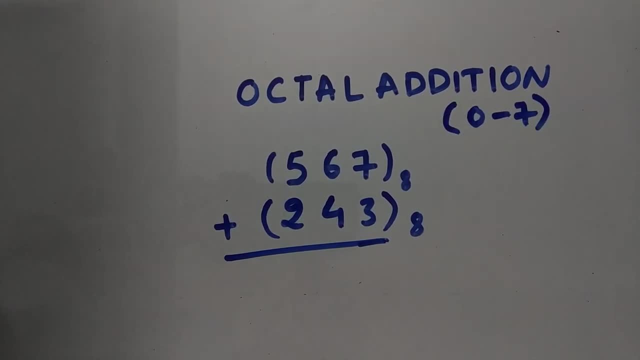 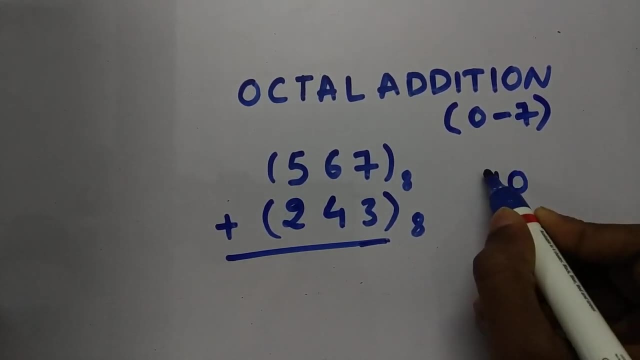 into octal. so now let's go into octal. 1, 7 plus 3 is 10, so that is in base 10, don't forget it, it's in decimal. now we need to convert into octal. so convert into octal divided by 8. so 8, 1, 0, 8 and 8, 2 is the. 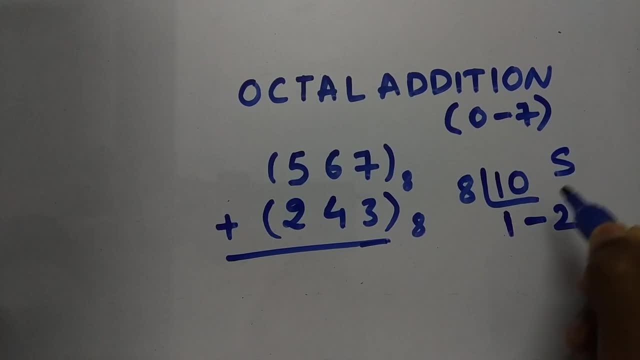 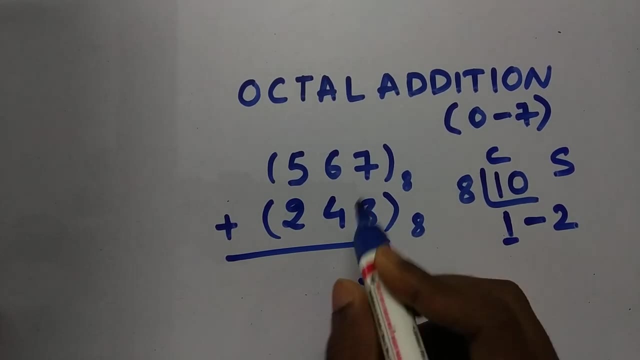 reminder. so this is the sum. don't forget, this is the sum and this one is carry, this one is carry. so now, sum, we can write over here: carry, we need to go for the next one, so it will be added over here. so now again, 6 plus 4 plus 1 is 11. 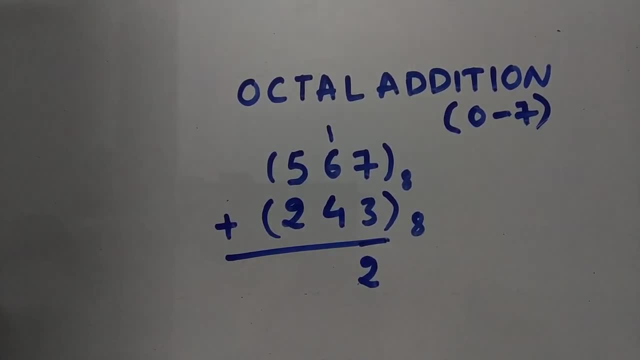 so 11. we need to convert into octal, so 8. 1 0, 8. the reminder is 3, so 1 & 3. again, 3 is the sum, 1 is the carry, don't forget this one. 3 is the sum, one is carry. so 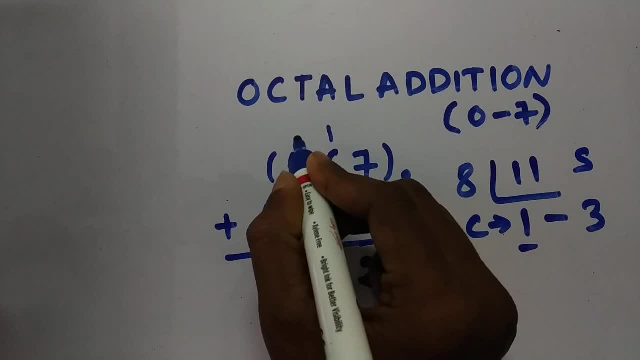 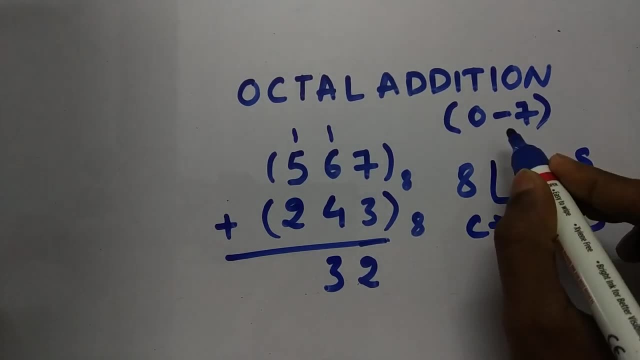 write 3 over here and carry 1 over here, so 5 plus 2 plus 1: 8. this is quite tricky. 8 doesn't fall under this. and the nth order over here, so 8 plus 2 plus 1: 8. this is quite tricky. 8 doesn't fall under. 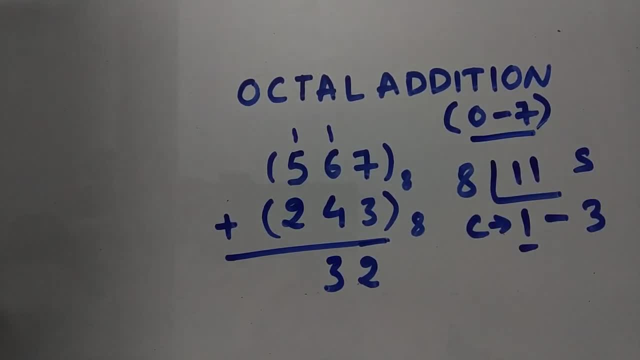 0 to 7, so we cannot represent 8 in octal addition, so we need to convert it again. so 8 and 8, 8, 1, 0, 1 and reminder is 0, so 0 and 1. so now, now carry is 1 over. 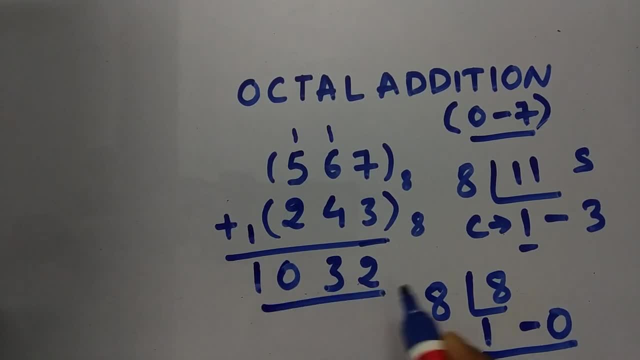 here. so 1, 0, 3, 2. so this is how we add two octal numbers. don't forget that, whatever we add, we are humans. we are addicted to decimal, so don't go for a decimal. we need to convert this decimal value into octal and then again do the. 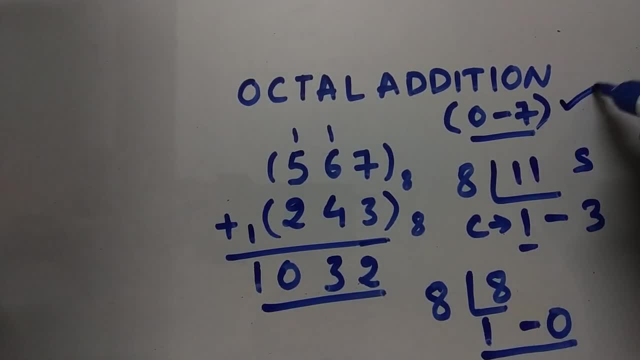 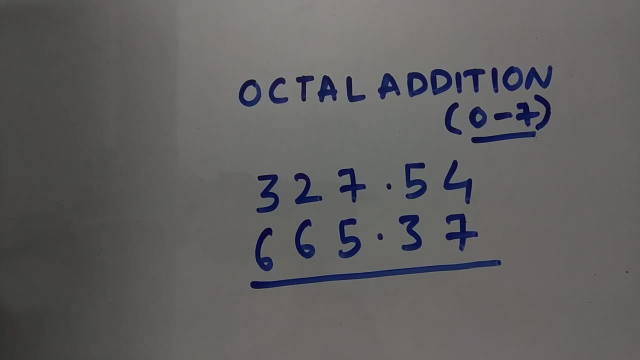 addition, don't forget that octal ranges from 0 to 7. let's take another example for your better understanding. so this is a example, so we are going to solve this. are octal numbers ok? so 7 plus 4 is 11, ok, 11. 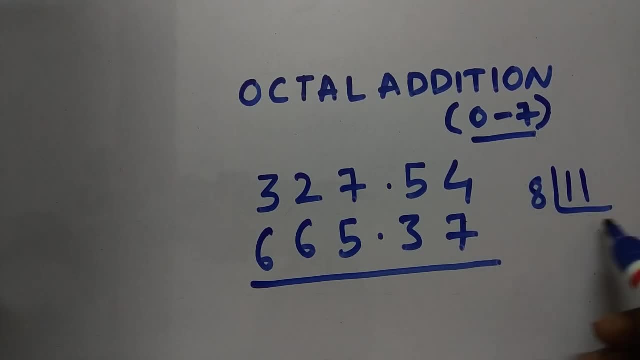 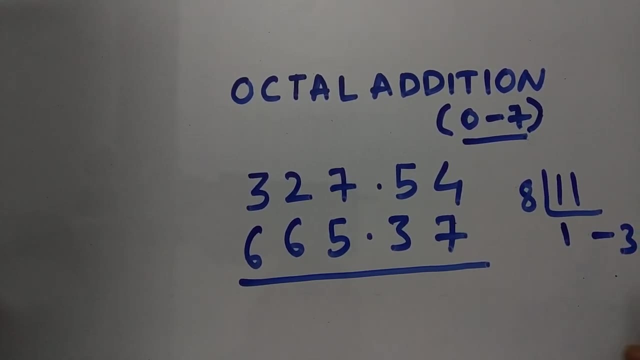 and we need to convert into octal. that is decimal, so we need to convert into octal. so 1 and 3. so 3 is there and 1 is the carry, so 3 is over here. 1 is carry, 5 plus 3 plus 1, 9. so again convert it. 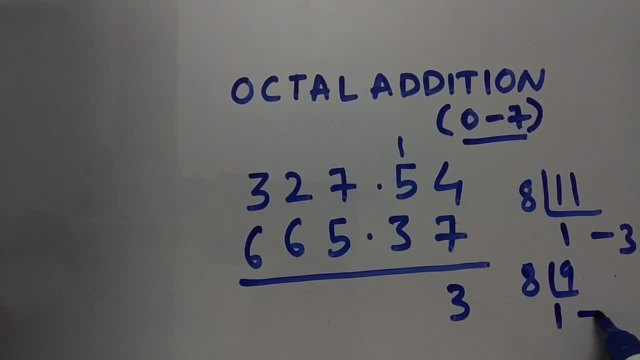 8 divide 9, so we'll get 1 and 1. so 1 is sum over here and this is carry and this is sum. don't forget that one. so now you get one over here, one over here. so now 7 plus 5 plus 1 is 13, so again, 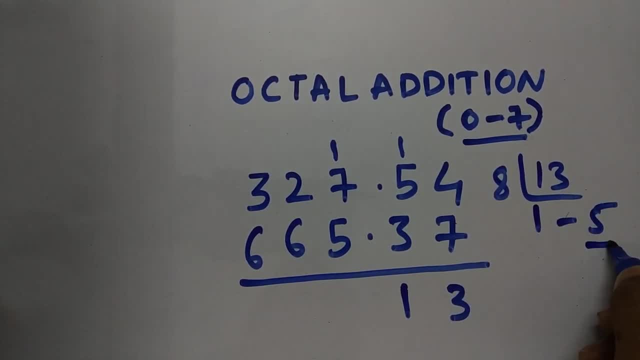 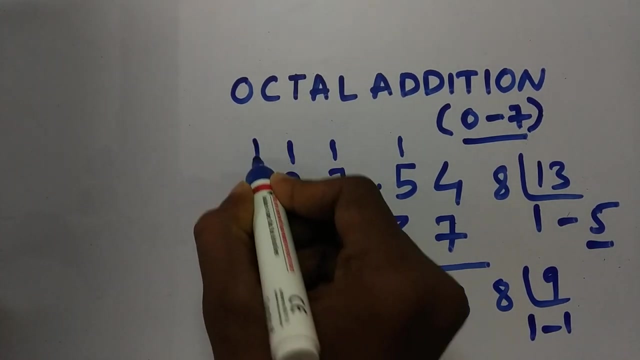 8, 1 and 5. so 5 is over here, 1 is carry over here. 6 plus 2 plus 1. 6 plus 2 plus 1 is 9. again, you know 9 is 1 and 1 because we have done it previously. so 1 again carry is 1. 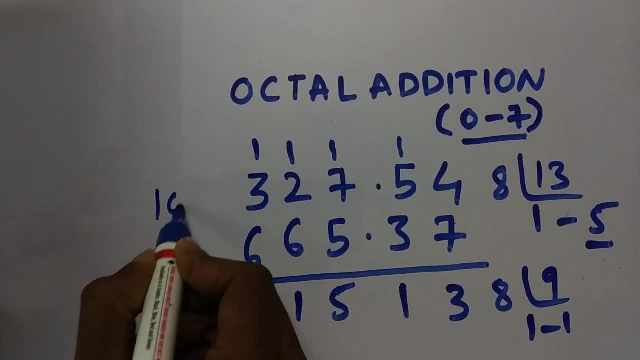 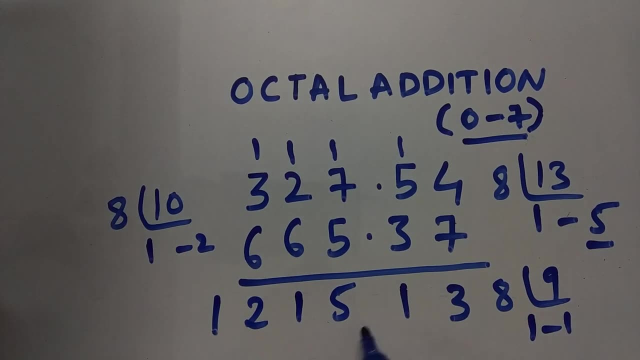 6 plus 3 plus 9, so it's 10, so 10, you can go by 8, 1 and 2, so here it's 2 and it's 1, so this is your answer. so this is your answer. so this is your answer in octo.